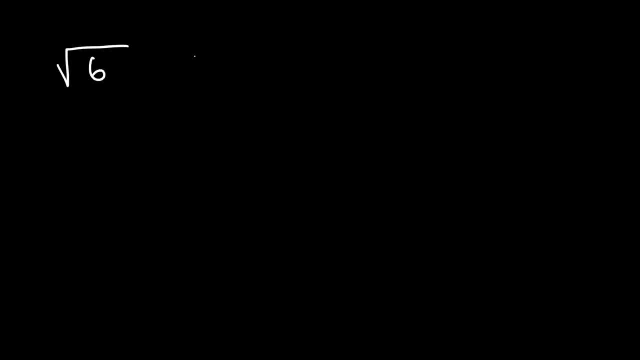 Now what about this example? What is the square root of 6 times the square root of 15?? So 6 times 15 is 90.. And we can simplify: root 90.. 90 has a perfect square in it, 9.. So let's break up 90 into 9 and 10.. The square root of 9 is 3, so the final answer is 3 root 10.. 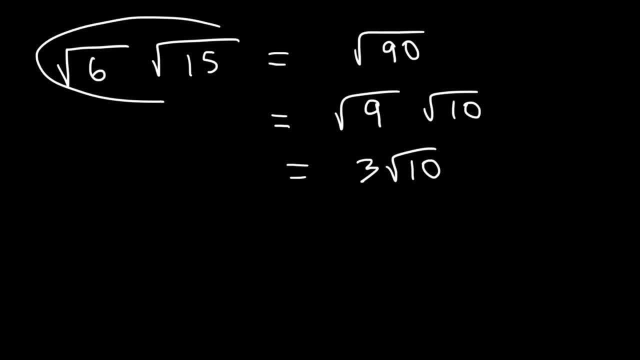 Now, granted, you can simplify it before you multiply. For example, we can rewrite 6 as 3 and 2, and 5, I mean 15- as 3 and 5.. The square root of 3 times the square root of 3 is simply 3.. And then we have root 2 times root 5, which we can combine as root 10.. So you can also do it this way. 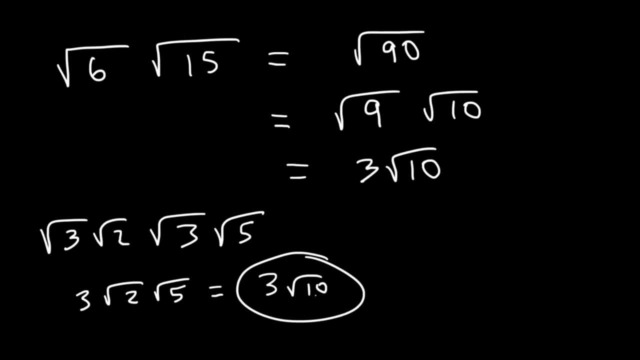 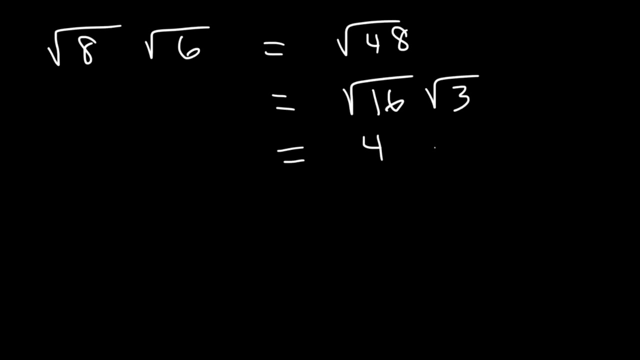 Sometimes it's better to simplify before you multiply if the number is too large. Here's another example: What about the square root of 8 times the square root of 6?? So we can multiply and say it's root 48. And a perfect square that goes into 48 is 16.. 48 divided by 16 is 3. And the square root of 16 is 4.. So the answer is 4 root 3.. 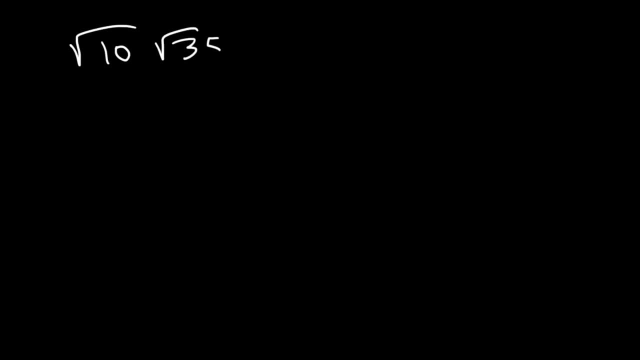 Now what about the square root of 10 times the square root of 3?? Now we can multiply and get 350, but is that the best way to approach this problem? 350 is a big number. What we should do is break down 10 into 5 and 2, and 35 into 7 and 5.. 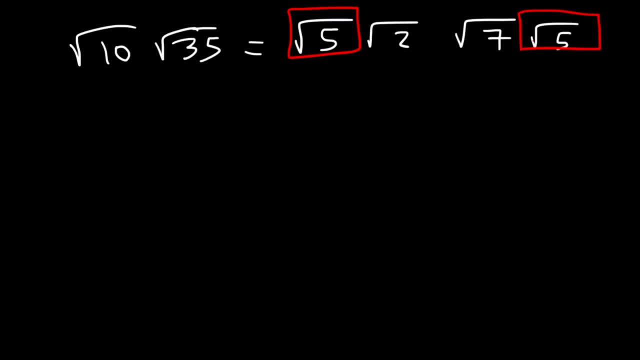 Now, because these two are the same, we can combine them: 5 times 5 is 25.. 2 times 7 is 14.. And the square root of 25 is 5.. So this is 5 root 14.. 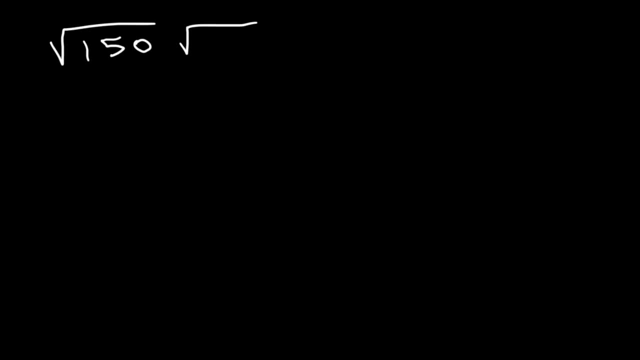 Try this one: 150 times 30. So we definitely don't want to multiply right now. We want to simplify before we multiply, Since this is going to be a very big number. 150 is basically 15 times 10.. 30 is 15 times 2.. 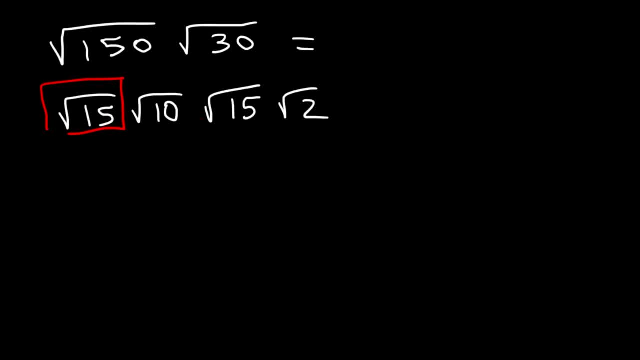 So these two, 15 times 15, that's 225.. And 2 times 10 is 20.. The square root of 225 is 15.. Now 20 has a perfect square in it. You can break it up into 4 and 5.. 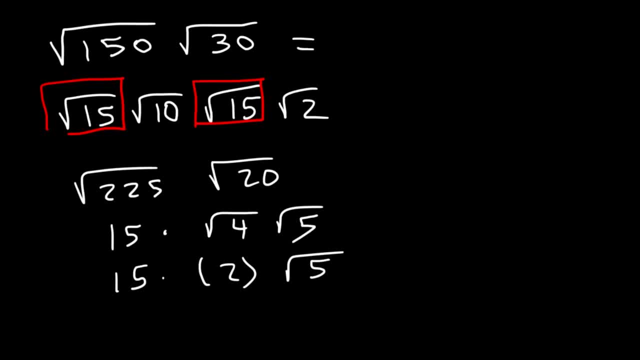 The square root of 4 is 2. And 15 times 2 is 30. So the answer is 30 root 5.. What about this one, The cube root of 18 times the cube root of 6.. So we can simplify first or we can multiply together. 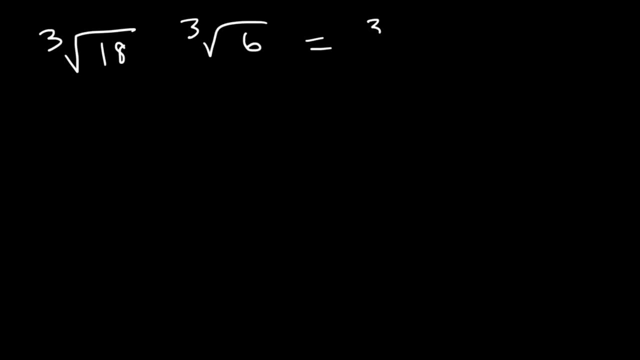 Let's multiply first 18 times 6, it turns out that it's 108. And a perfect cube that goes into 108 is 27.. 27 times 4 is 108. And the cube root of 27 is 3.. 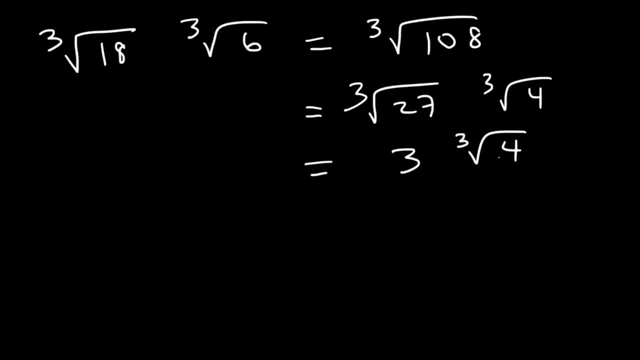 So the answer is 3 root. It's 3 cube root, So the answer is 3 root of 4.. Now we can also get the answer doing it this way as well: 18 is basically 9 times 2. And 6 is 3 times 2.. 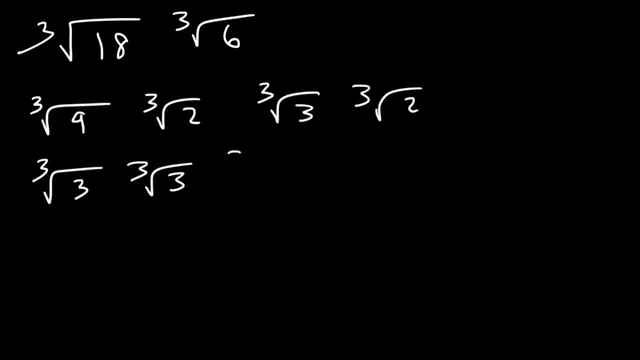 And 9 is 3 times 3.. Because the index number is 3, to get a number outside of the radical we need 3 of those numbers. Notice that we have 3 cube root 3's, So that is just going to come out as 3.. 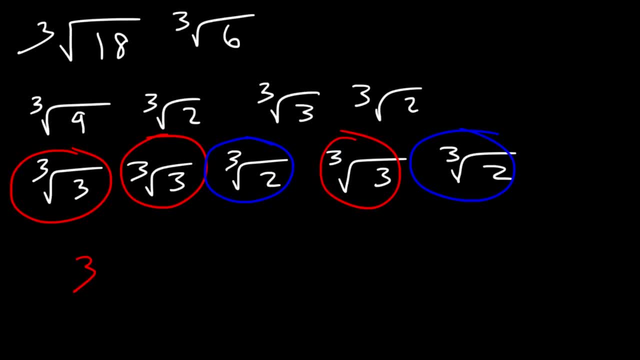 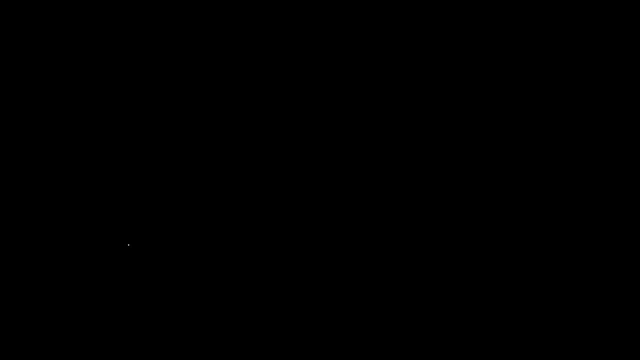 We don't have 3 2's, So we can multiply the 2's 2 times 2 is 4. And so that's another way we can get this answer. Now, what if we have variables? What is the square root of 18x cubed? 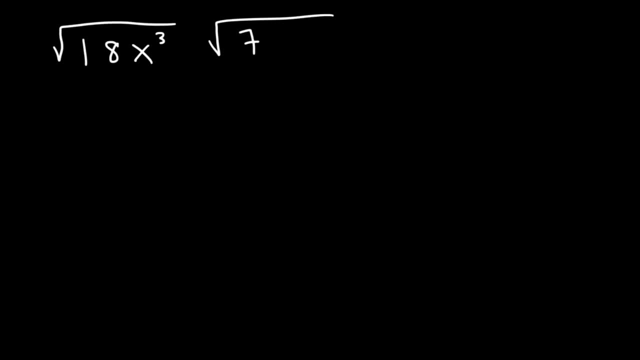 times the square root of 3?? What is the square root of 72x to the 5th? Feel free to multiply those radical expressions and simplify Now what I like to do: separate the numbers from the variables. 18 is basically 9 times 2.. 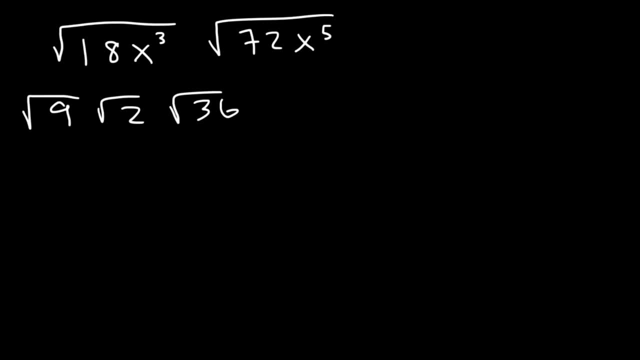 And 72 is 36 times 2.. And then x cubed times x to the 5th is basically x to the 8th. The square root of 9 is 3,, the square root of 36 is 6, and root 2 times root 2, that's the square root of 4, which is simply 2.. 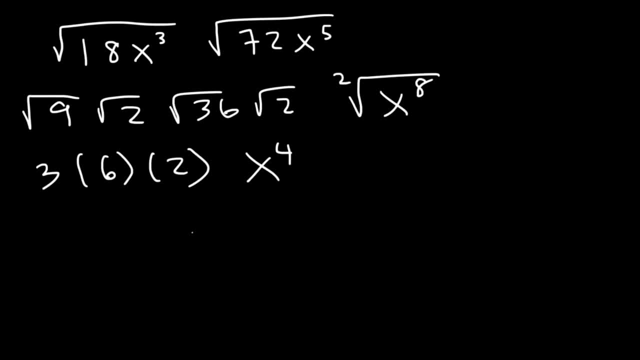 And now, the square root of x to the 8th is x to the 4th. 6 times 2 is 12,, 12 times 3 is 36,, so the final answer is 36x to the 4th power. 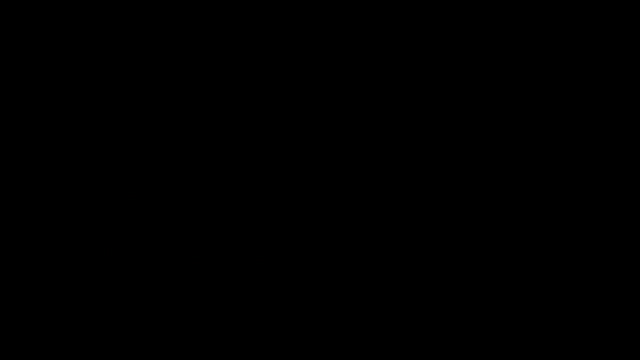 Now what about this one? The cube root of 12x to the 5th y to the 3rd times, the cube root of 6x to the 8th y to the 7th. So 12 is basically 2 times 2.. 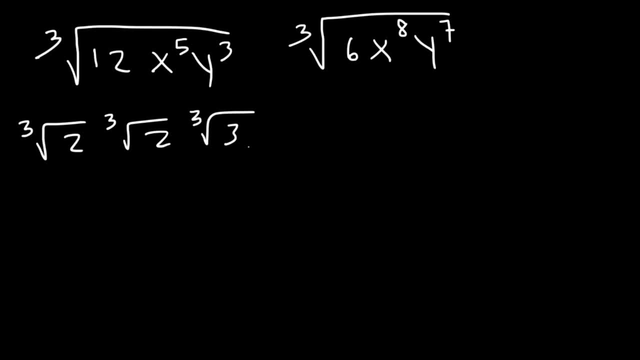 Times 3.. 2 times 2 is 4, times 3 is 12.. And 6 is 2 times 3.. Now x to the 5th power. times x to the 8th power, That's going to be x to the 13th power. 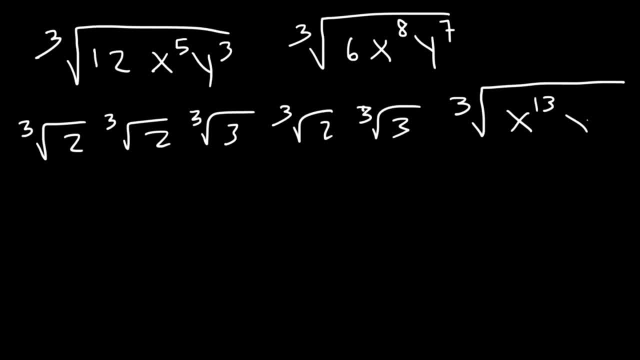 And y to the 3rd times, y to the 7th. 3 plus 7 is 10.. So notice that we have three 2s: 2 times 2 times 3.. 2 times 2 is 8.. 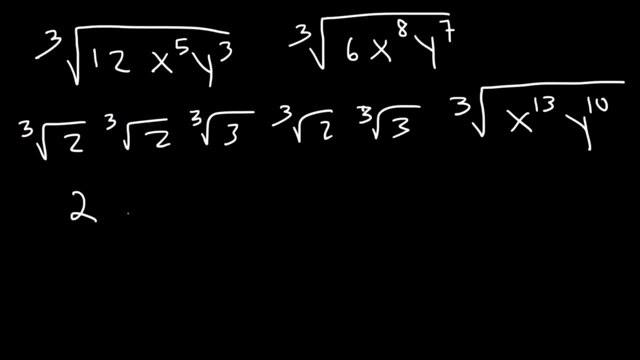 The cube root of 8 is simply 2.. We can't take the cube root of 9.. So right now I'm just going to combine it and leave it as the cube root of 9.. Now, what about the cube root of x to the 13th? 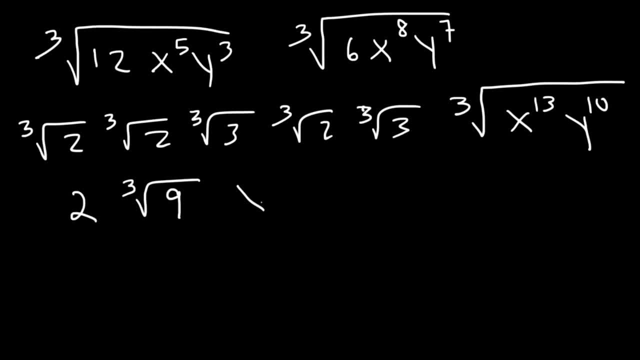 3 goes into 13 four times And 3 goes into 10 three times. Now, 3 times 4 is 12.. So there's going to be 1x remaining, And 3 times 3 is 9.. 10 minus 9 is 1.. 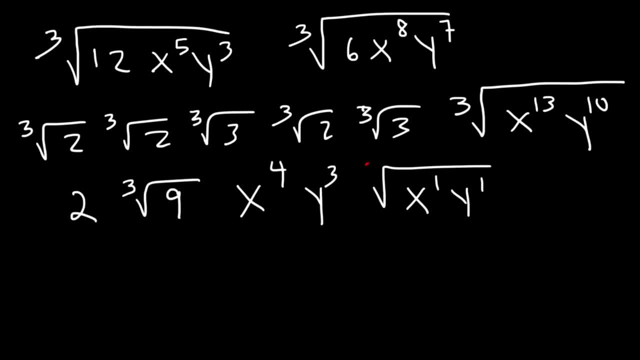 So there's also 1y value remaining. Now we can combine these two. So the final answer is 2x to the 4th power, y to the 3rd times the cube root of 9xy. That's as far as we can go.